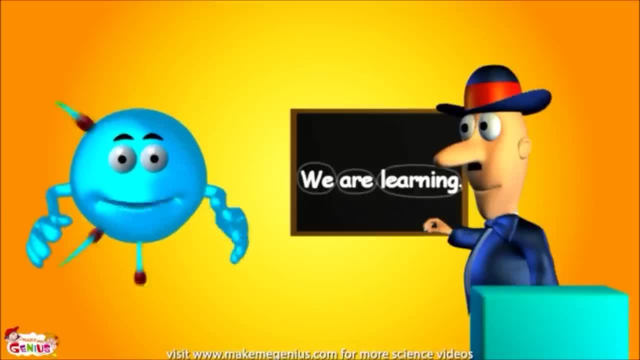 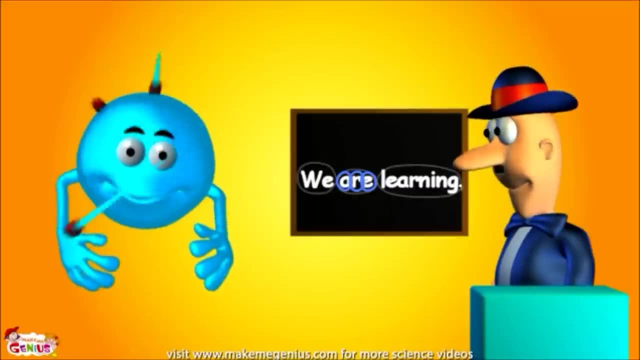 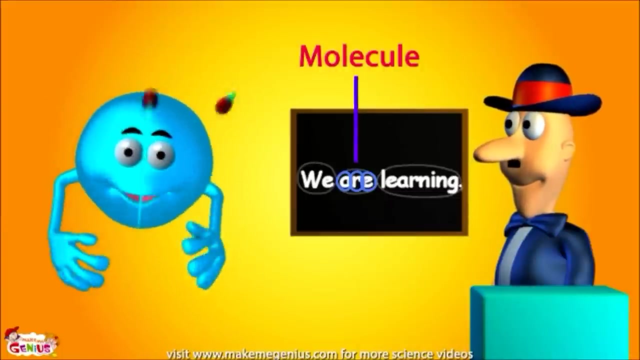 Now let's take a word and circle all the letters of R with some other color. Very good, You see, this sentence is made up of words, but words are made up of letters, So letters are the smallest units of a sentence. Similarly, everything is made up of molecules, but molecules are made up of atoms. 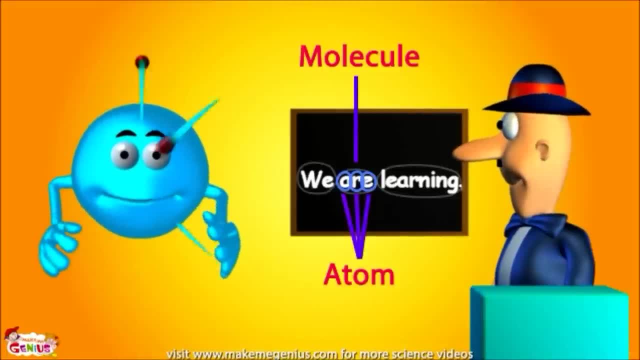 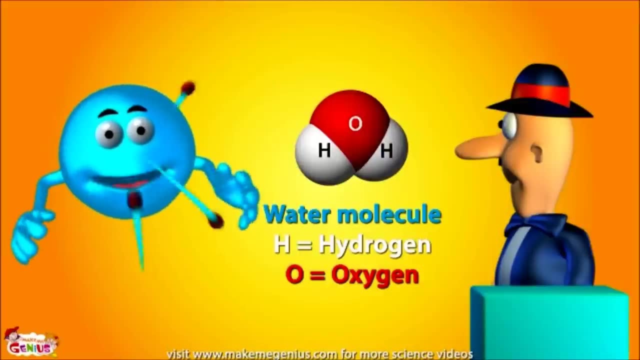 So atoms are the smallest unit of everything. Look at this, See, water is made up of water molecules, but water is made of atoms. There are two atoms of hydrogen and one atom of oxygen in each water molecule. So when atoms join together, they form a molecule. 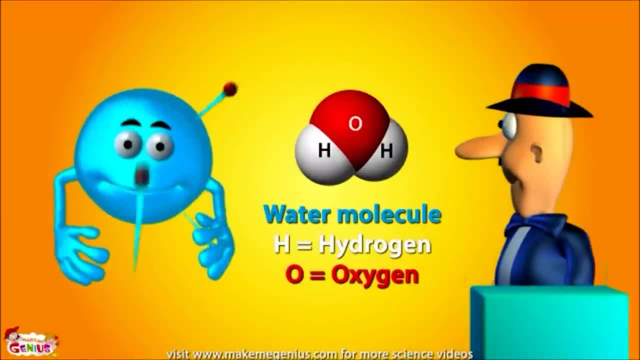 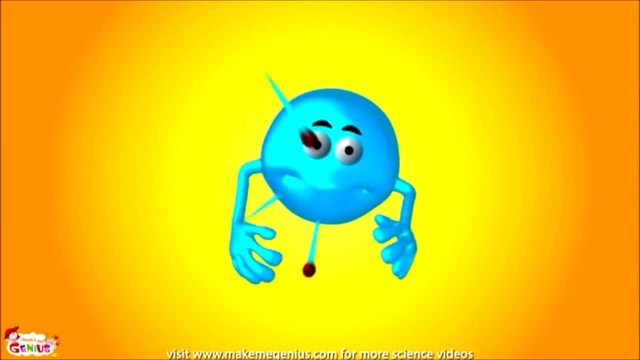 And when molecules join together, they form a thing. So now you understand Good. So now, friends, now I would show my body, Yes, I would show different parts of my body. In the center of an atom, there is the nucleus. 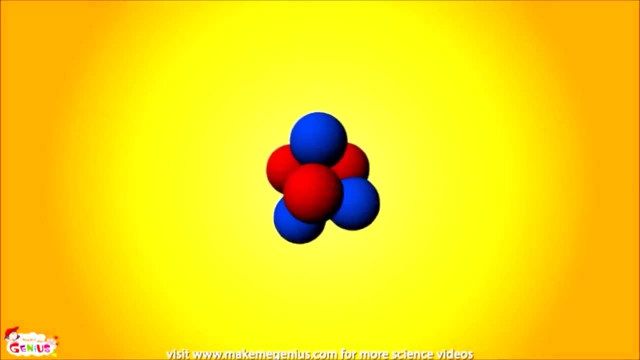 It is made up of even smaller parts. These are called protons and neutrons. Each of these protons carries a positive electrical charge. The neutrons are equally as heavy as protons but don't carry any electrical charge. So the nucleus of an atom is positively charged due to protons. 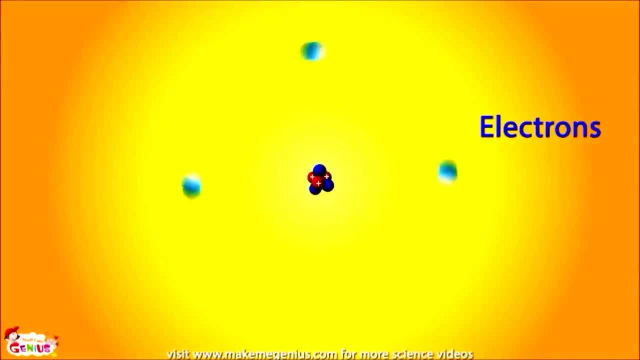 Now electrons are outside the nucleus, They are orbiting around the nucleus. The electrons carry a negative charge. The total negative charge of electrons is equal to the positive charge of the nucleus. So in total an atom is neutral. The positive charge of the protons is neutralized by the negative charge of the electrons. 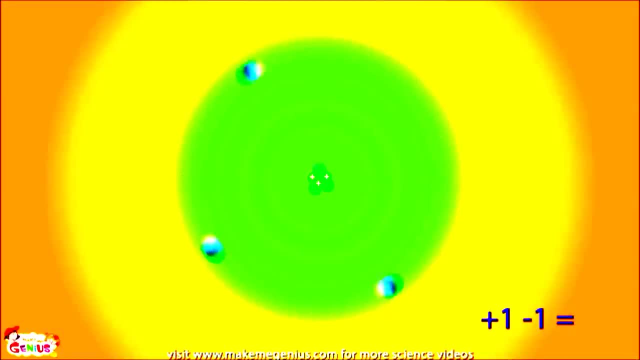 So it is like plus one is neutralized by minus one and overall charge of an atom becomes zero. The electrons are moving outside the nucleus at a very high speed. Can they run away from the nucleus? No, they can't run away. Every atom has the same number of protons, electrons and neutrons. 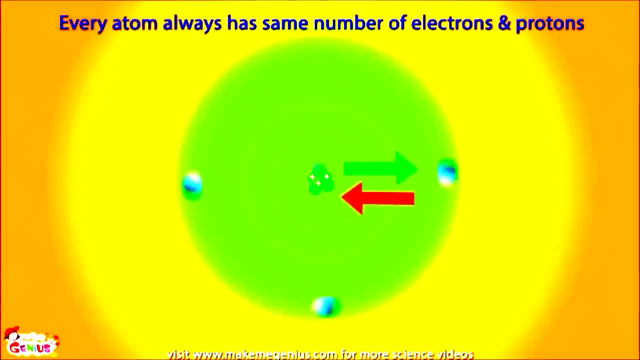 So there is an attraction between equally strong negative and positive charges. Due to this attraction, electrons can't run away, as positively charged protons keep them pulled towards them. Hope this is all clear to all of you. Otherwise you can always go back and see it again.